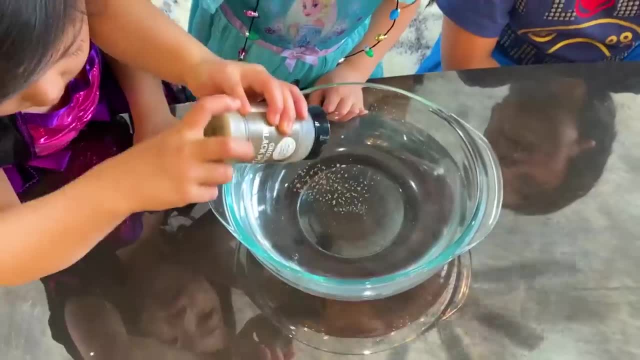 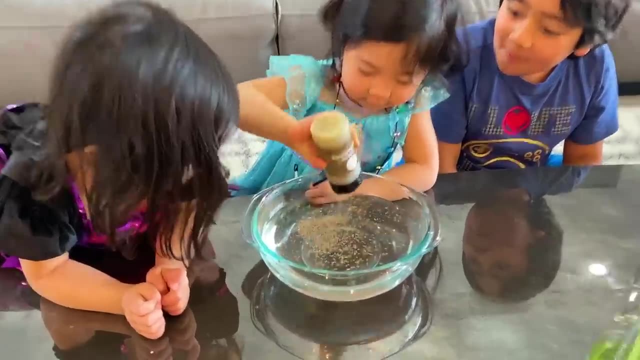 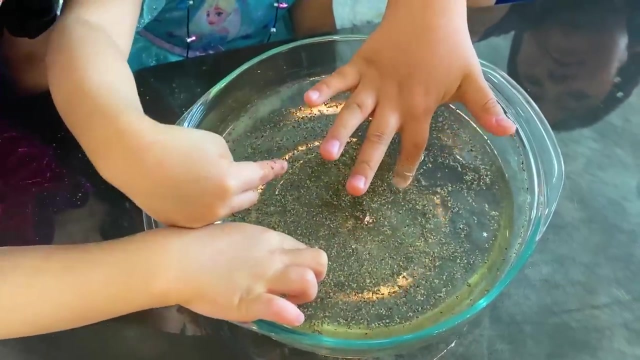 Okay, so sprinkle some peppers in there. Do I do it? Yeah, take turns, Sprinkle more. You can do a lot more than that. What? There you go. You're doing a lot. Next step is I want you to take your little finger and dip it into the pepper water. 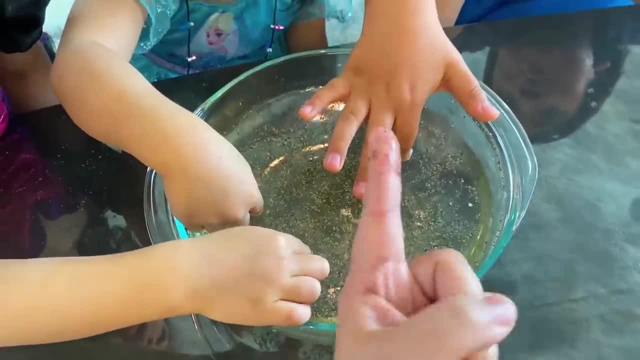 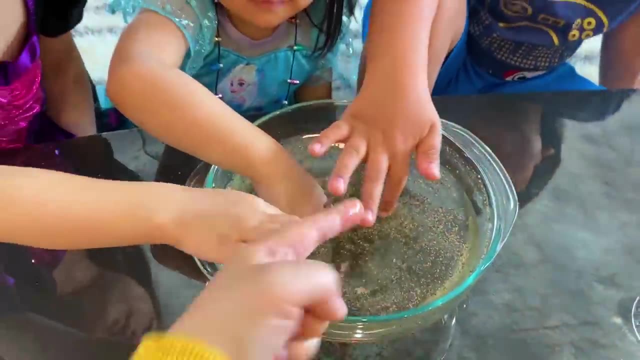 Now I want you to pretend these pepper water are germs. What happens when you take your hands out? Oh no, There's germs. Yeah, you see. And if you touch it there's germs. right, Look, there's germs on you. 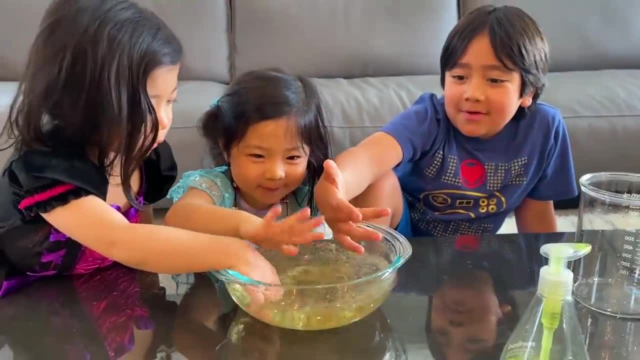 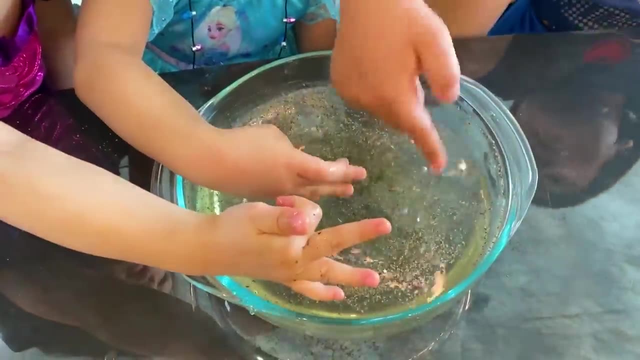 There's germs on me. I know, You see the germs, Yeah, Okay. So here's why It's important to wash your hands. You ready? Yeah, Okay. so that's what happens without soap: It just sticks on your hand, right. 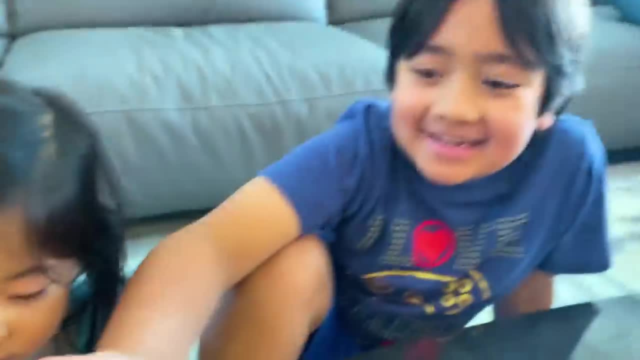 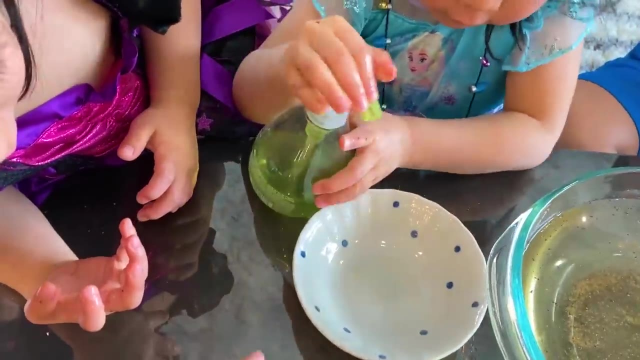 Ooh, germs everywhere, Ah, Ah. Next, I want you to squirt soap into here. I want to do it, There you go. Can you squirt some soap into there? I hold for you, There you go, Good. 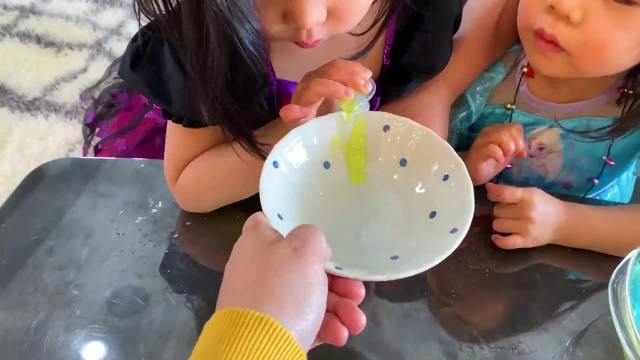 All right, okay, turn. There you go. All right, Okay, that's a lot. Here's what I want you to do: Take your little finger And then dip it into soap. There you go, Dip in a lot. 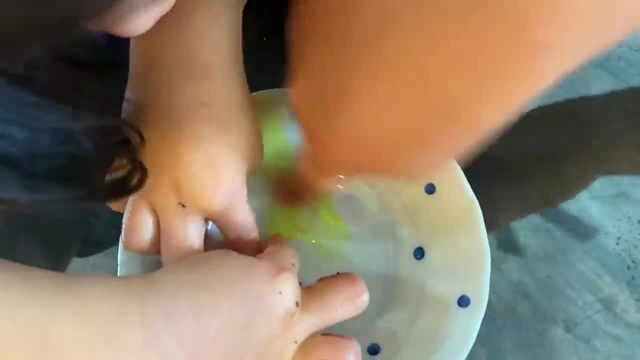 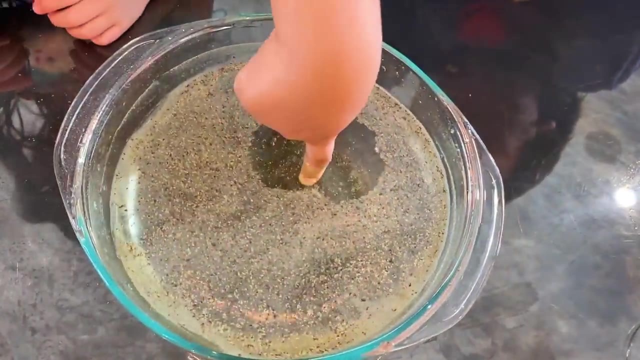 Okay. So this is why soap is important. First, Ryan's going to do it. Okay, Go ahead. Whoa, What happened? The pepper's going away from the soap. I know It looks like the pepper's running away from the soap, right? 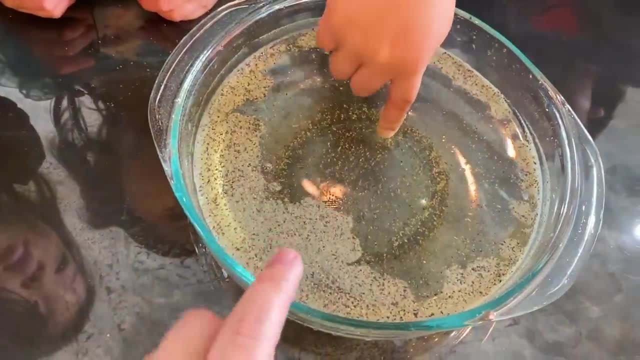 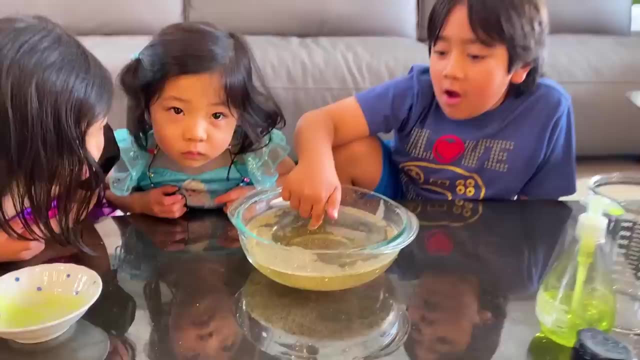 Yeah, So think about it. So if these are like germs and bacteria, when you put your hands in soap and wash your hands right, All the germs and bacteria are no longer on your hands. Yeah, They're running away. 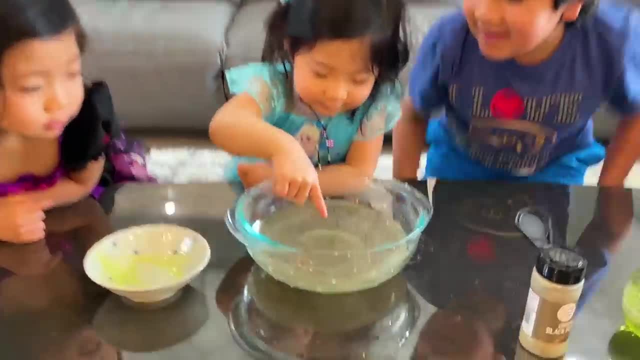 Can I try? Yeah, of course It's my turn. Whoa, That's so cool. See how it's running away. Whoa, That's so cool. Whoa, All right, Kate, you want to try now? 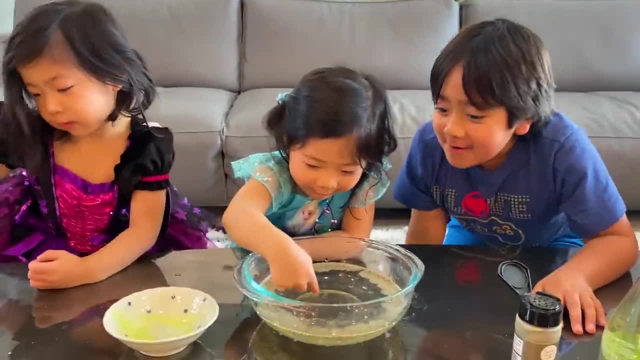 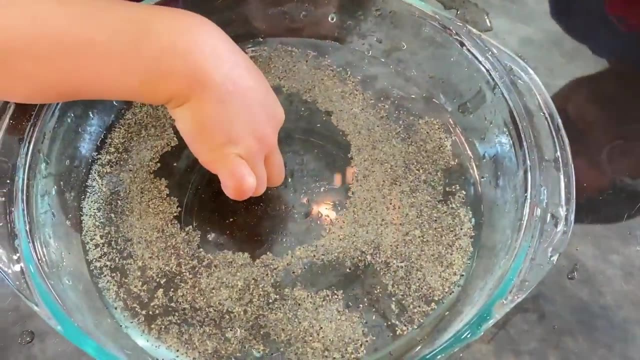 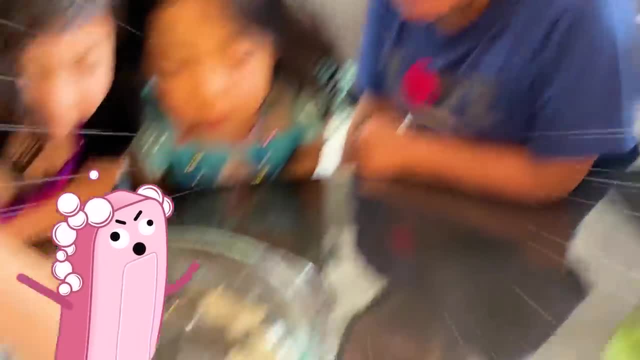 Yeah, It's like: oh no, soap, Ah, Ah. That's why it's very important to wash your hands. Now we're going to do it with glitter, Yeah, So you guys can each take a glitter or a share. 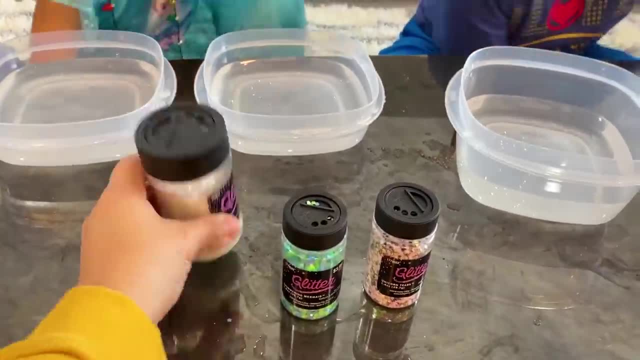 I want this glitter And put it into water and pretend these are germs. There you go, I'm putting a lot, You're putting a lot of germs. Yeah, I'm going to put a little bit. Okay, A lot of germs for Emma. 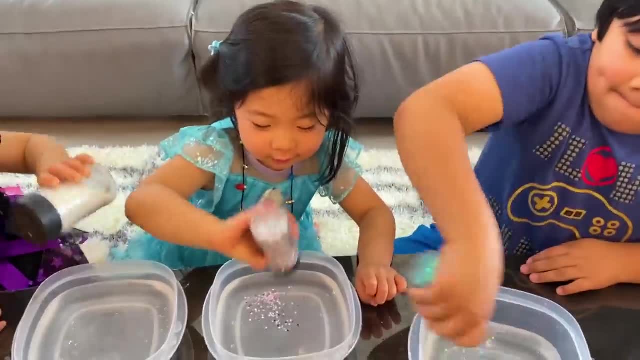 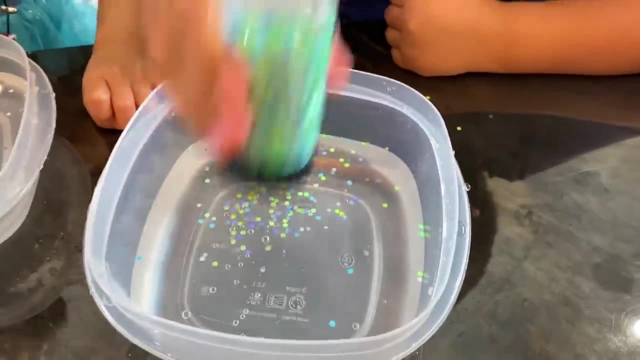 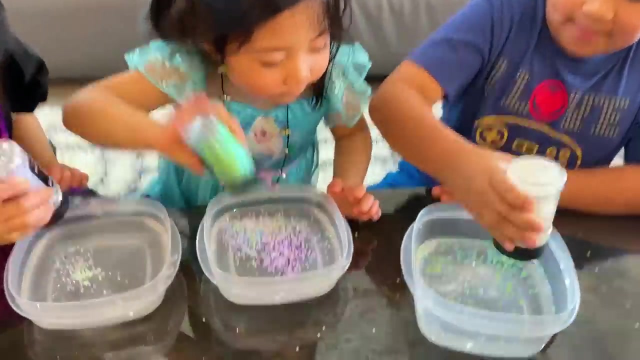 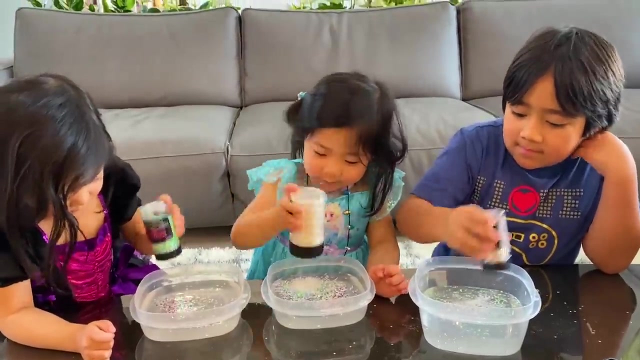 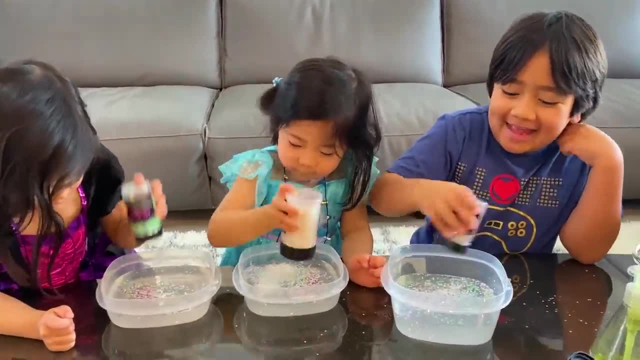 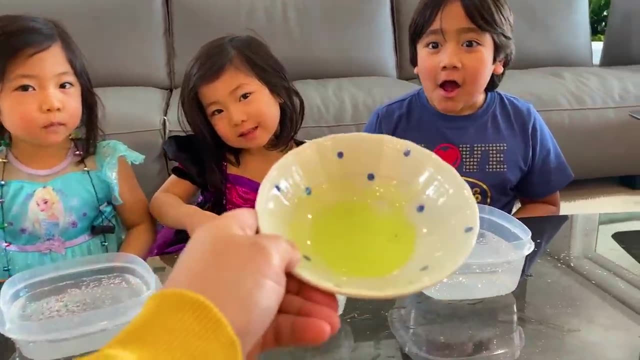 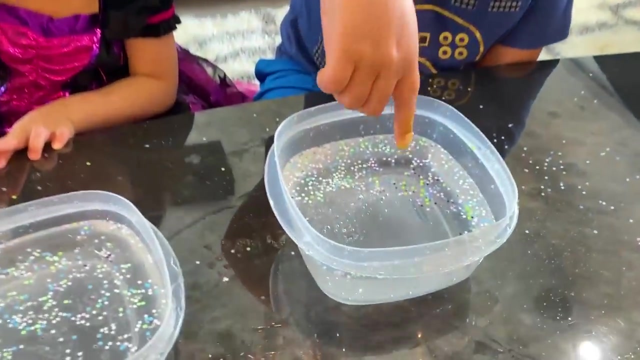 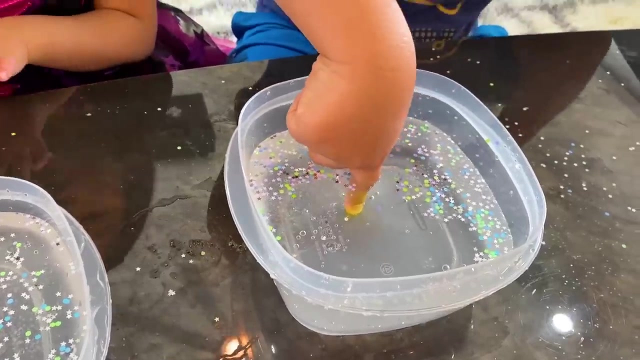 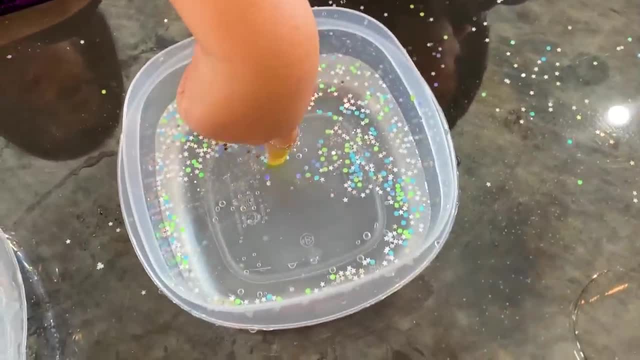 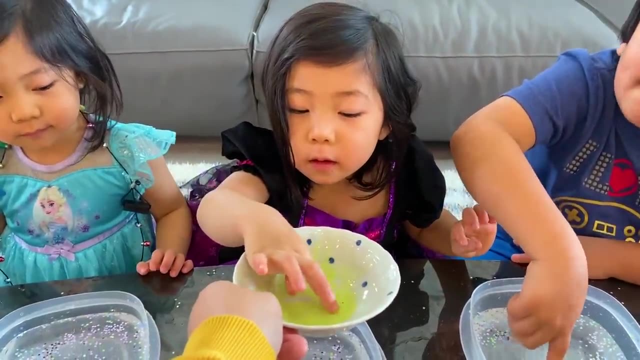 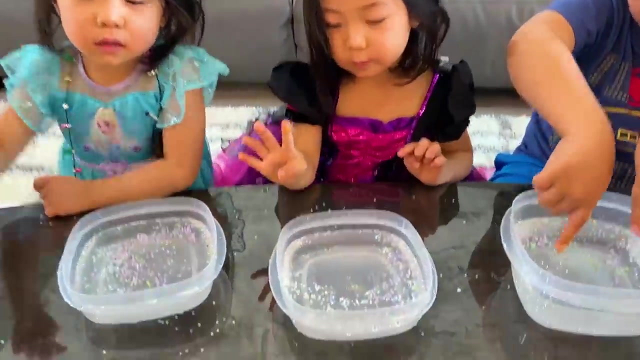 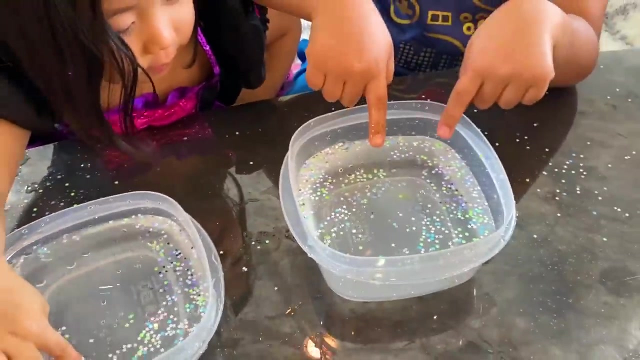 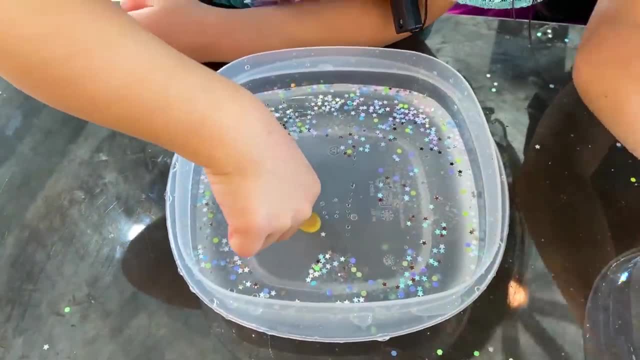 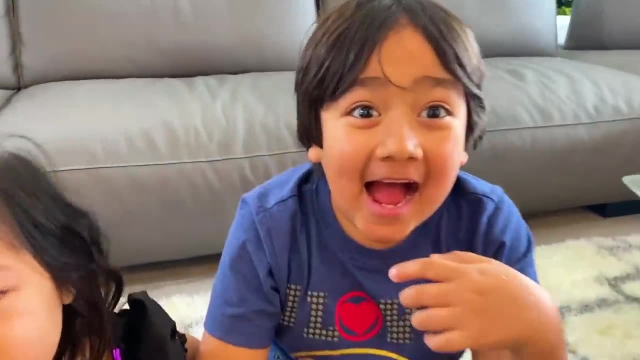 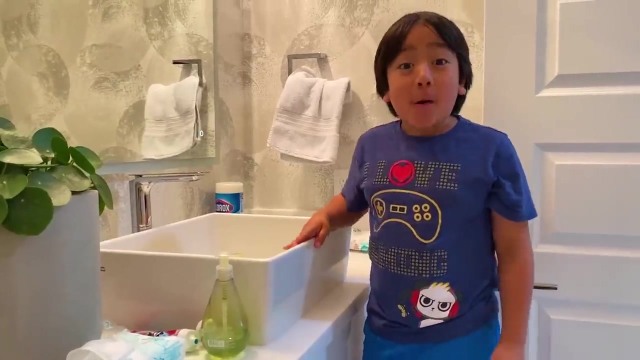 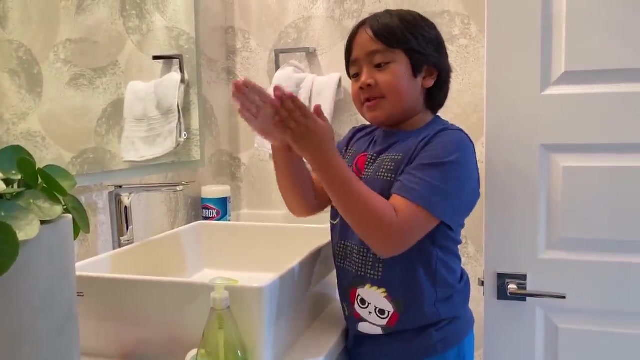 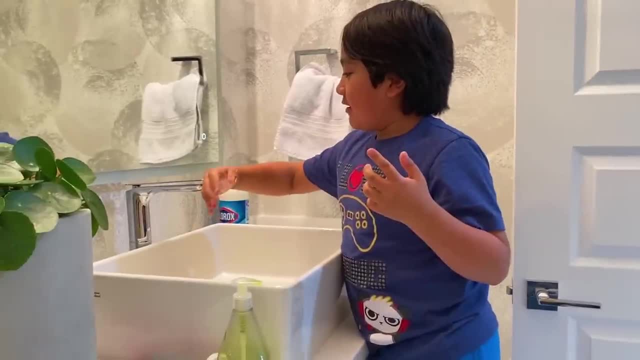 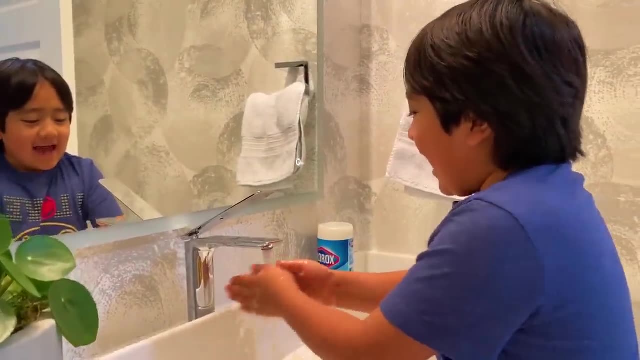 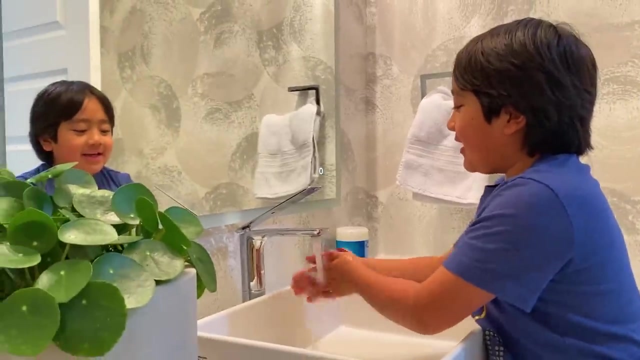 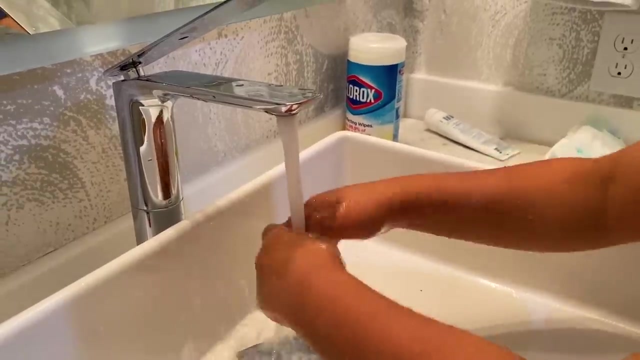